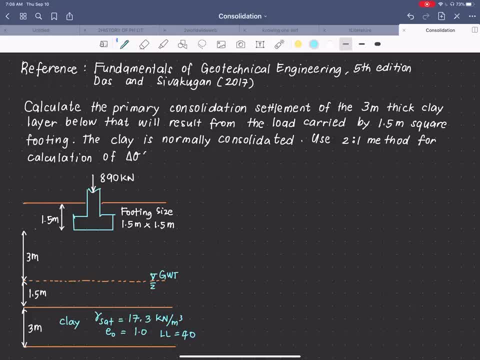 So we want to calculate the settlement of this clay layer. that will result from the load carried by 1.5 mth. So we have a square footing here which has a section of 1.5 by 1.5 mth. 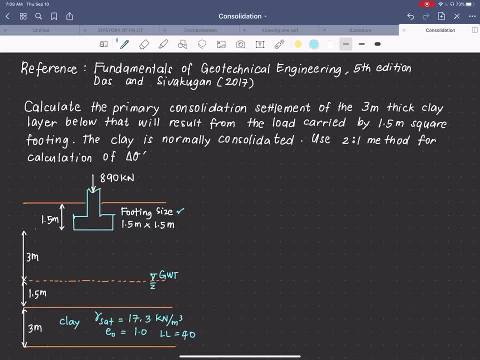 And the load carried by this footing is 890 kN. The soil above our clay layer is sand, So we have here a dry sand Having a dry unit weight of 15.7 kN per cubic meter, While below the groundwater table, which is located 4.5 m below the ground surface. 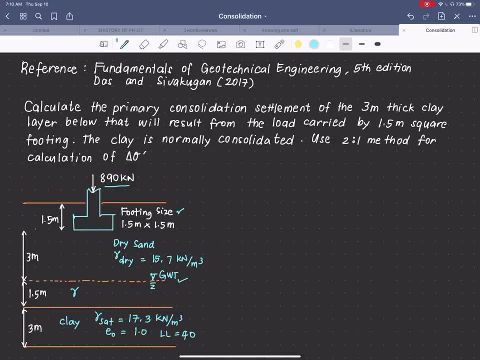 And this is the saturated sand having a saturated, the submerged, rather having a saturated unit weight of 18.9 kN per cubic meter, And the clay is given to be normally consolidated And we are Asked to use the 2 is to 1 method for the calculation of delta, sigma prime or the given surcharge. 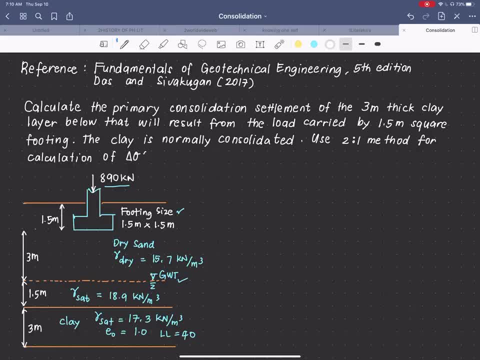 All right. So let us try to look at the given data, or given values, So as to calculate the primary consolidation for this normally consolidated clay. If we are going to look at the formula for a normally consolidated clay, That is equivalent to, We have 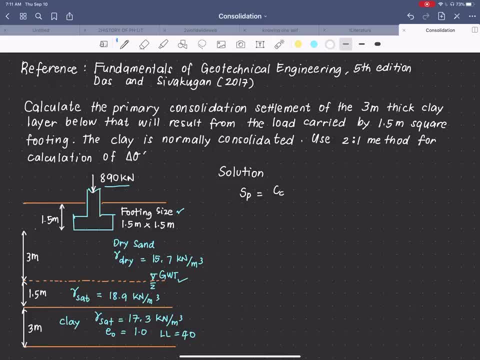 C sub C. H over 1 plus E sub O. Log of Sigma, not prime, plus delta sigma. prime divided by sigma, not prime. So that is the equation to calculate the primary consolidation. Let us see if all parameters are given. So C sub C. 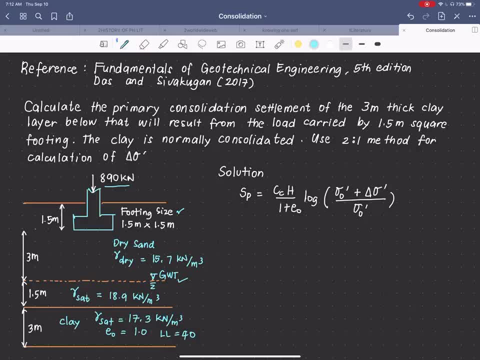 C is not given, but we can actually calculate it given the values Like E, sub O or the institute void ratio, as well as the liquid limit. We can use the Skempton's parameter or formula. So H is given to be 3 meters. 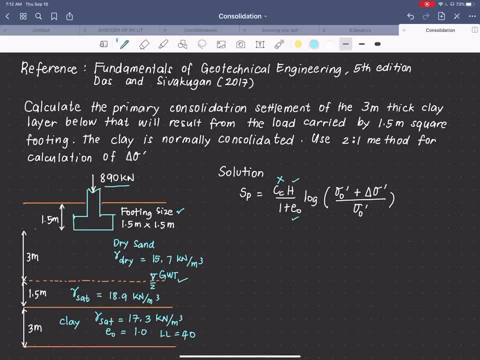 The void ratio institute is given, And then The, The effective stress, can be calculated. Okay, but it's not given yet. Okay, this one is not given also, And this one is not given yet. So let us try solving first the C sub C. 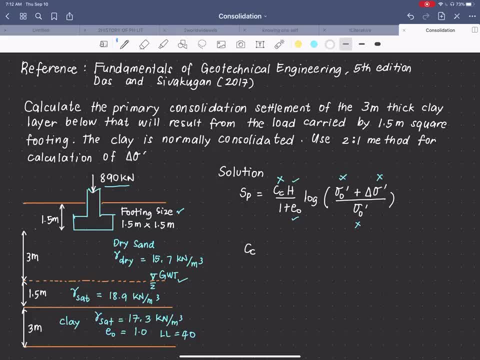 Or the compression index. So compression index can be calculated using the Skempton's formula of point Zero zero nine Multiplied by The liquid limit minus Ten, And this is equivalent to: This is assuming And disturbed sample: Point zero zero nine. 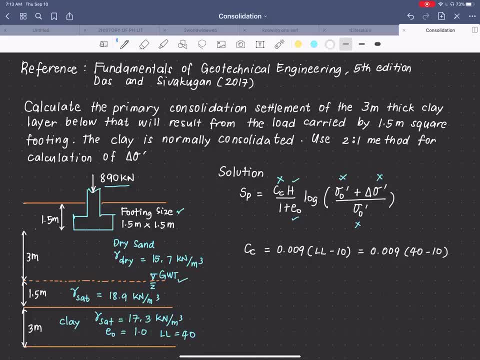 Forty Minus ten. Our liquid limit is forty. So C sub C can be Calculated and that is equal to point Twenty seven. Okay, our H is three meters, so that is given, that that's right. Or let us use three thousand. 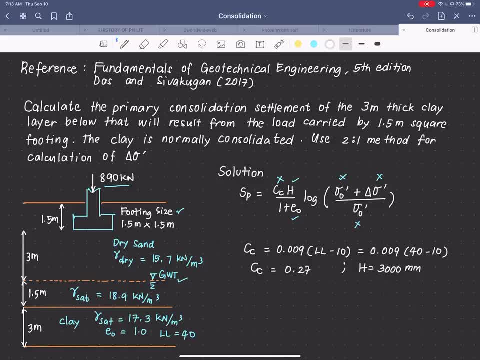 Millimeter Is of all is One. And let's solve now for The Preconsolidate, sorry, the overburdened pressure or the effective stress At the center of the clay layer. So at the center of the clay layer we have. 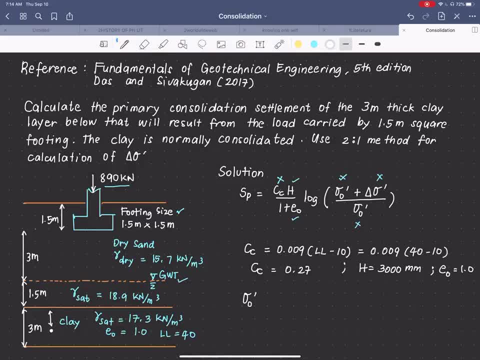 Here A thickness of One point five Meters. Okay, So, from the ground surface, Let us start With The first layer, And the first layer is the dry sand. So we have Gamma dry Of sand Multiplied by 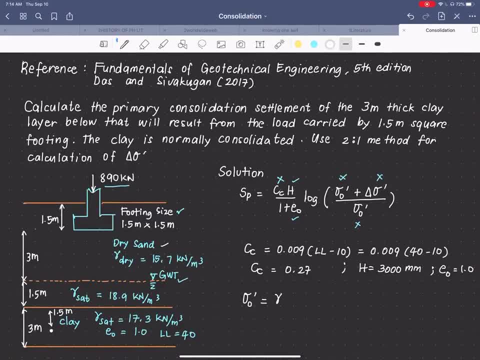 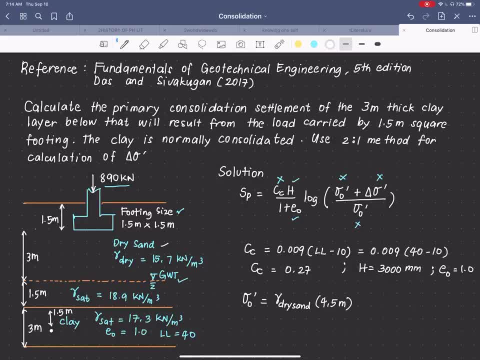 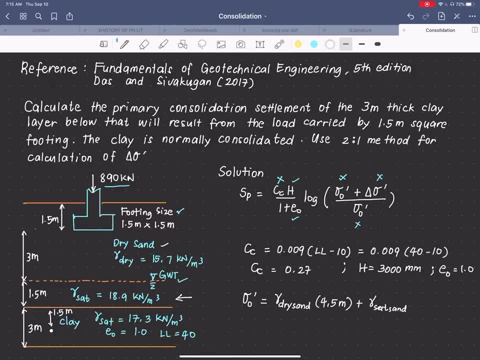 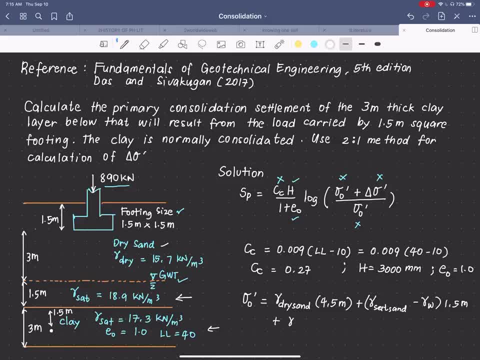 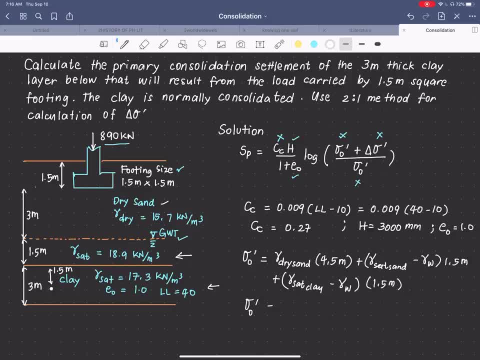 Minus, substitute and plug in the values, we have. gamma dry: the unit weight of the dry unit weight of sand is 15.7 kilonewton per cubic meter multiplied by 4.5 meters, plus the saturated unit weight of sand, which is 18.9 minus the. 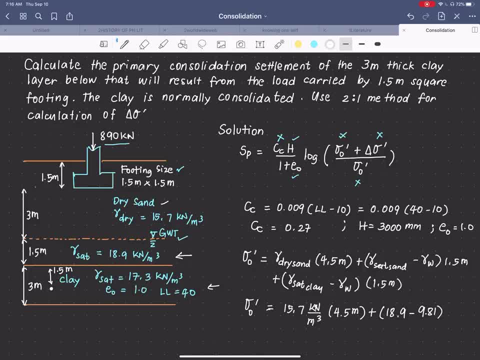 unit weight of water: 9.81. this is again kilonewton per cubic meter times 1.5 meters, plus saturated unit weight of clay, which is 17.3 minus the unit weight of water, 9.81 can kilonewton per cubic meter, and then we have 1.5 meters. 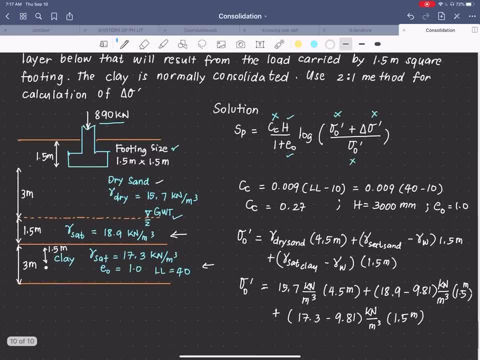 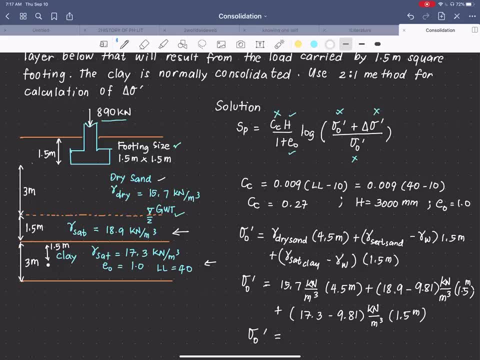 okay. so if you are going to calculate the effective stress, that would be equal to effective stress at the center of the clay layer. that is equal to 95.52 kilonewton per square meter. okay, so we already have this. we can now remove this. this is already known. 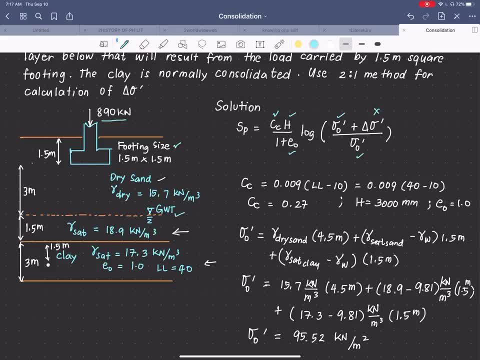 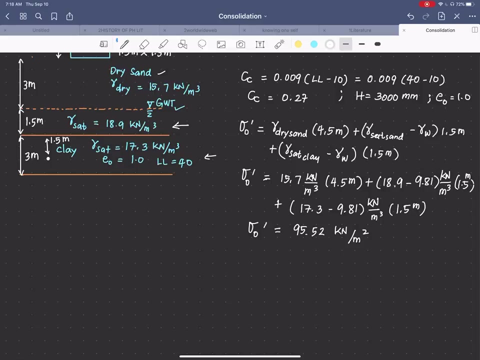 okay, this is already known, these three values, and so we just need to calculate the surcharge or the Delta Sigma Prime, which will use. the two is to one method, the two is to one method is an approximate method to calculate the surcharge and we have a formula for that. 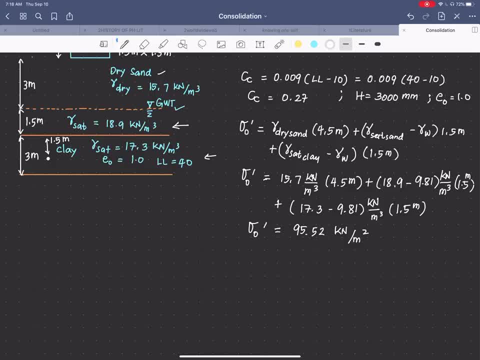 to determine the surcharge. this is equivalent to Q times B times L times B times L, B plus Z multiplied by L plus Z. or this is also equal to Q capital by B by L. oh sorry, this is also equal to Q by d plus Z and L plus Z. what is the difference? this one is in. 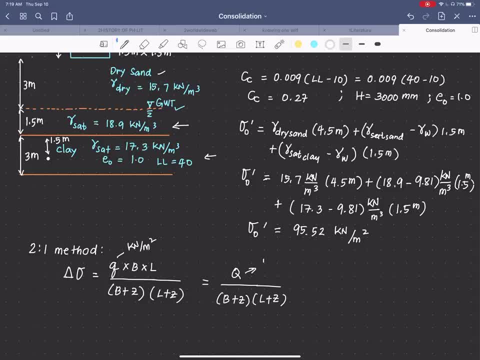 kilonewton per square meter. this was. this is in kilonewton, so this is the applied load, or the load carried by our foundation and, in our case, load carried by the file will be Fth by ad1 number, seven times zero, three times Fd: as6nicas1,ž. 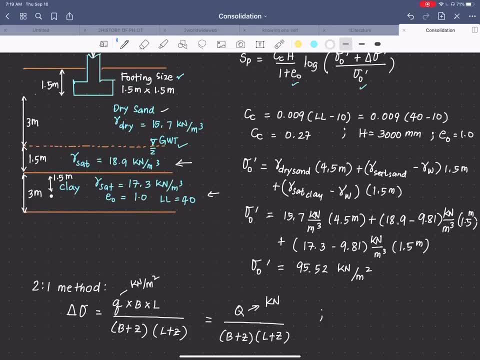 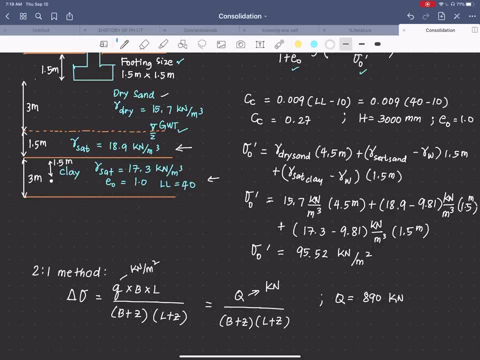 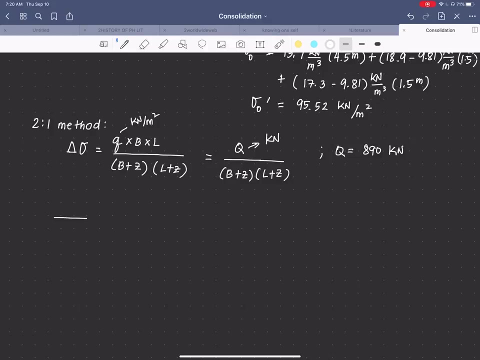 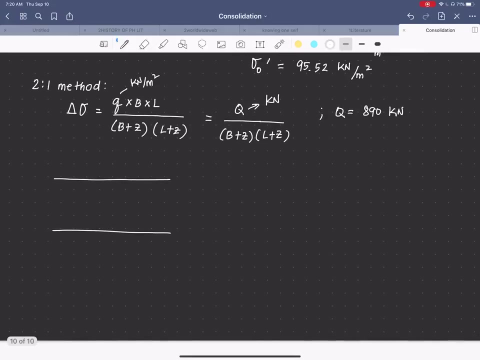 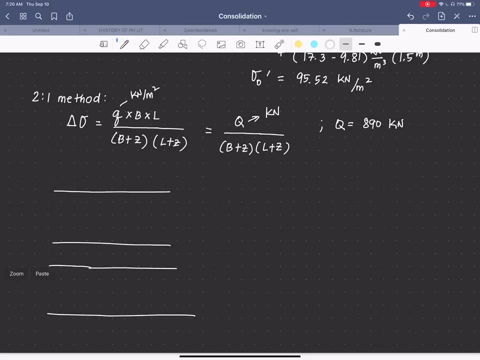 foundation is 890 kilonewton. so to get the Delta Sigma at the center of the clay layer you have to use a 2 iso 1 method or the trapezoidal. let me just draw it again. we have here, and this is our clay layer. 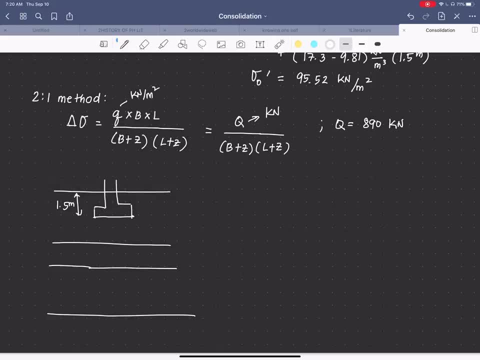 this is 1.5 meters and then, if this is our create layer, okay, this one is 4.5, or that we just read from here. here we have three meters, then we have another 1.5 meter here and we have here the clay layer, which is three meters, and we have a Q equals 890 kilonewton. so to 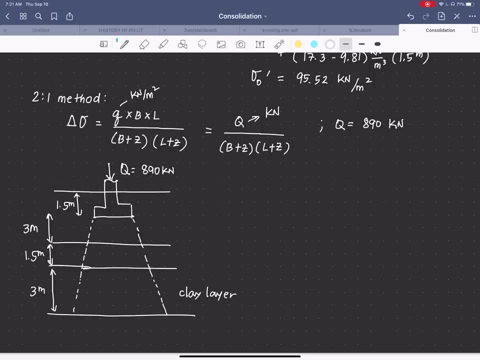 get the average Delta Sigma at the center of the clay layer, you have to use the formula Delta Sigma average. you have to use the Simpson's rule. this is the Simpson's rule, which is Delta Sigma on top, or this one that plus forms four times the Delta. 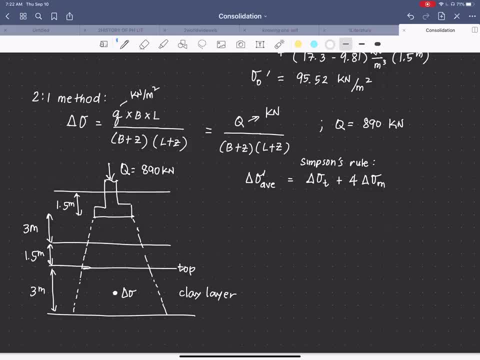 Sigma at the mid. this is the meat of your clay layer, plus Delta Sigma at the bottom. so this is the bottom divided by six. okay, so if you look at this value, you already have this. Q, B and L are the section of our clay layer, our footing foundation, and since this is a 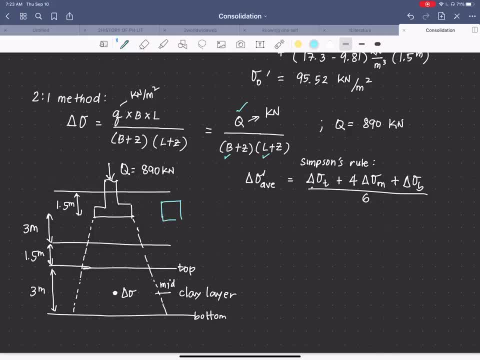 square footing and we are given a one point five by 1.5 meter. so B is equal to 1.5 and C is equal to 1.5 meter. also to this, to our given, while the Z value is the distance from the bottom of the clay. 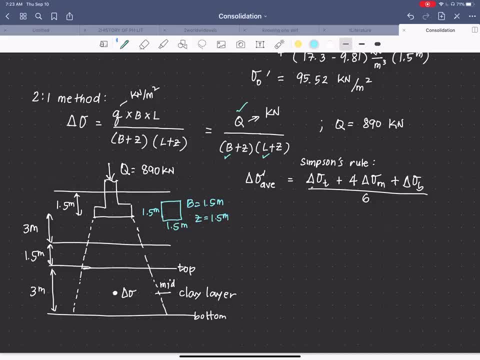 layer, sorry, the distance from the bottom of the footing foundation up to the point wherein we want to get the surcharge or the Delta Sigma. so, since we want to get the Delta Sigma at the top, so this is Delta Sigma top. here we have the Delta Sigma mid and delta Sigma mid and delta sigma on each extension of this tray and 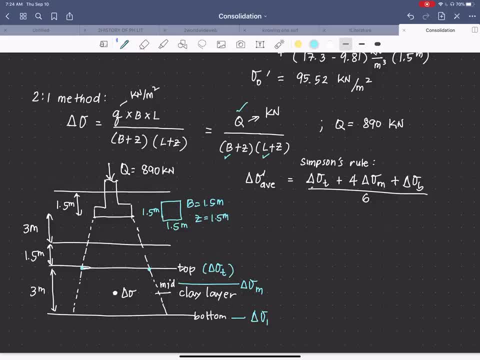 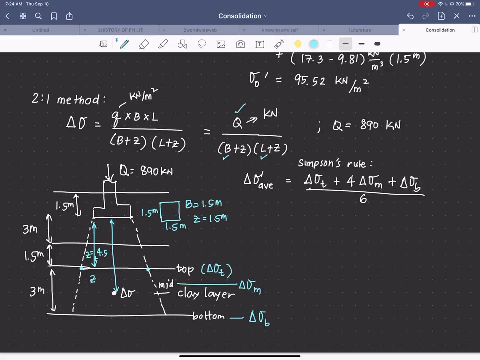 and this is a delta sigma bottom, and so the Z values here are. we have here 4.5 for the top. let me write C and another C for the. this is top, and then C mead is equal to four point five plus three, which is six meters. 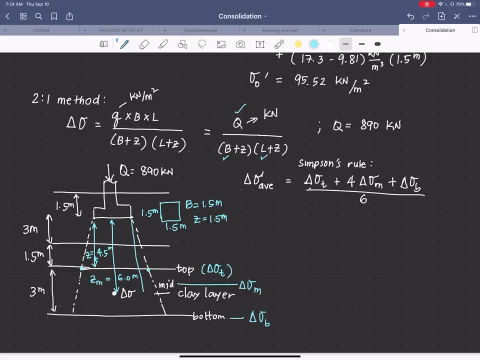 and at the bottom we have here Z at the bottom, which is equal to seven point five meters. all right, so we just simply use this equation. all the values are given already, and so let's solve for the Delta Sigma. at the top we have Delta Sigma. top is equal to. 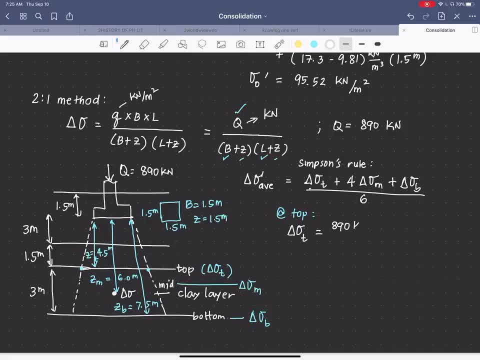 Q, which is 890 kilonewton, divided by B, which is 1.5, plus the C at the top, is four point five. this is to be multiplied by L is also one point five, plus C. that is also four point five. so we get here. 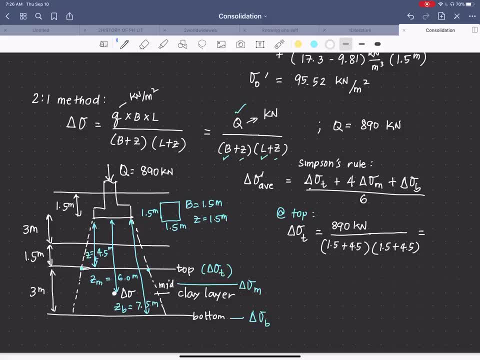 this is the firstиваем we can calculate. then, how many meters we're going to calculate in the nuevas like, if we are tohistology, and this is all this is in meter slopes, din Newton. we can calculate in k, helping many of per meter or square meter. okay, then we have at the mid of the clay layer is 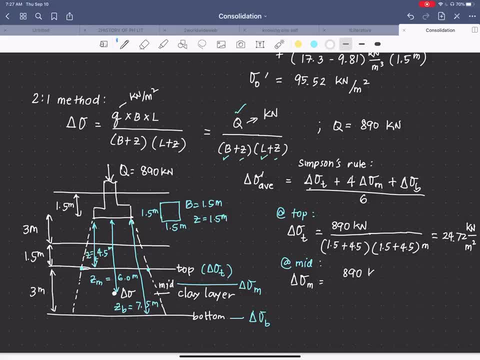 equal to still 890 kilonewton, but this time our B is still 1.5, but the C is already 6 meters, and then we have 1.5 plus 6 meters. so for this data we can get a value of Delta Sigma equal to. 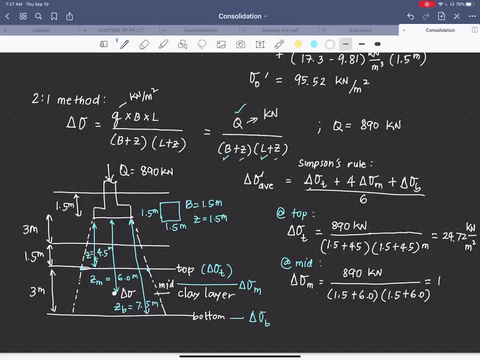 15 point 80 to kilonewton per square meter. so this is effective. and lastly, at the bottom we have Delta. Sigma at the bottom is equal to 890, kilonewton divided by 1.5 plus Z at the bottom is 7.5. so 1.5 again plus 7.5 and we get. 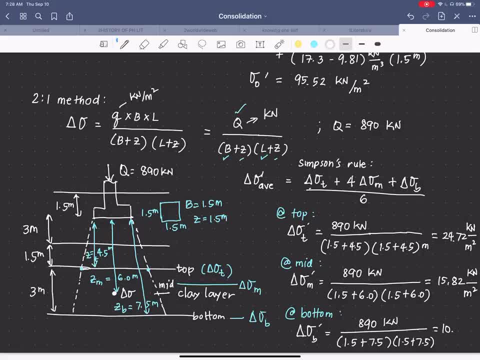 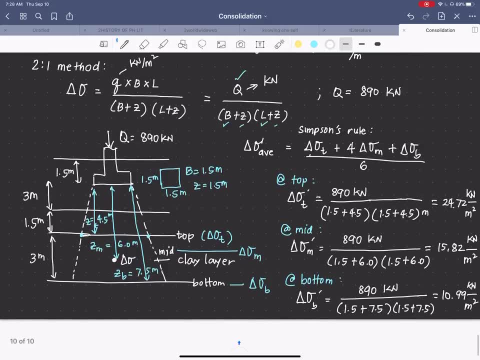 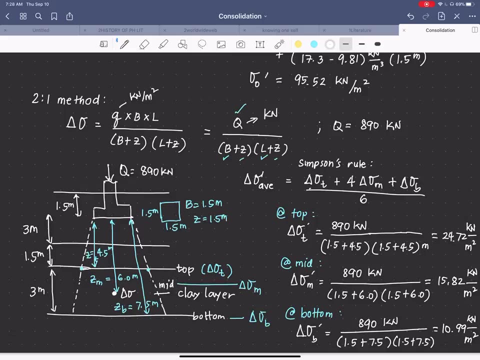 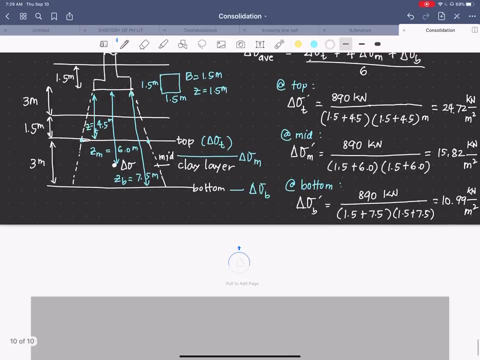 a value of 10 point 99 kilonewton per square meter. okay, and so, after having the Delta Sigma at the top, at the mid and at the bottom layer of the clay, we can now use the Simpson's rule to solve for the average. so Delta. 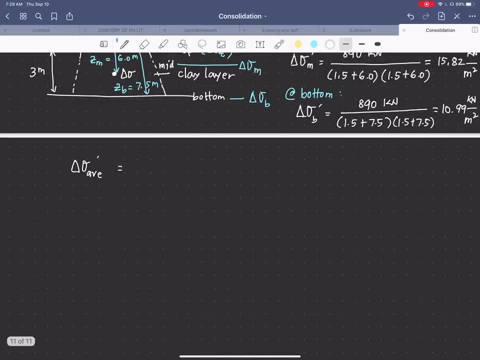 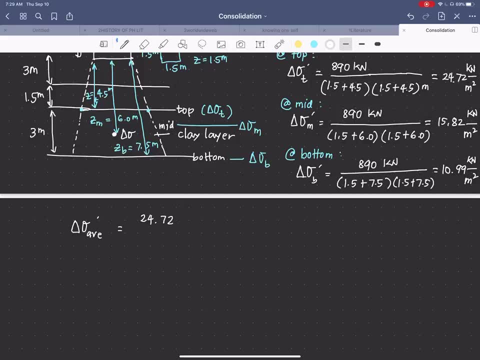 Sigma at the bottom is equal to 10.99 plus the middle medium of the clay layer is equal to. TVs is equal to. we have 24.72 plus 4 by the mid of four point fifteen point eighty two plus the bottom 10 point 99 divided by six. 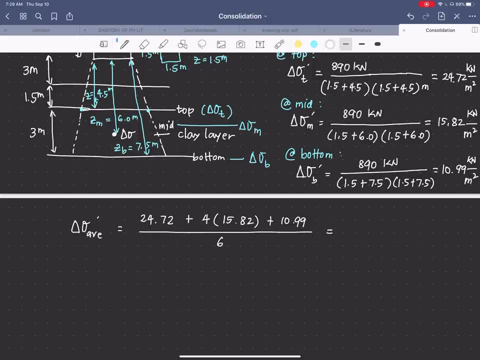 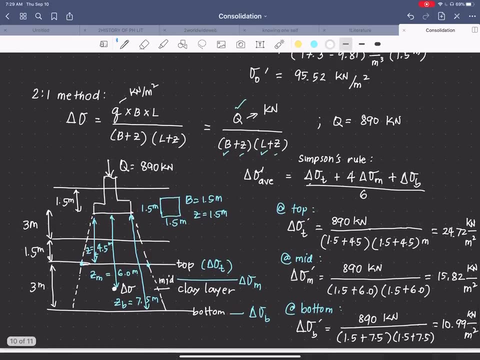 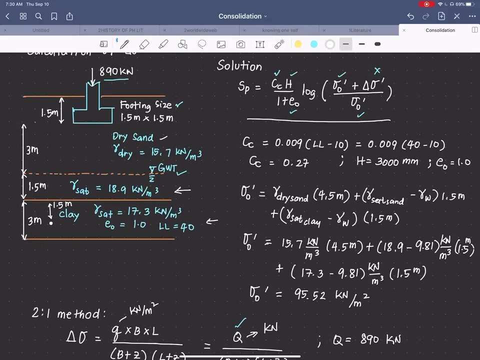 And so if you calculate, the delta sigma is equivalent to 16.5 kilonewton per square meter. And so all the parameters now are given. We can now calculate for our primary consolidation settlement. So let's try to plug in values. 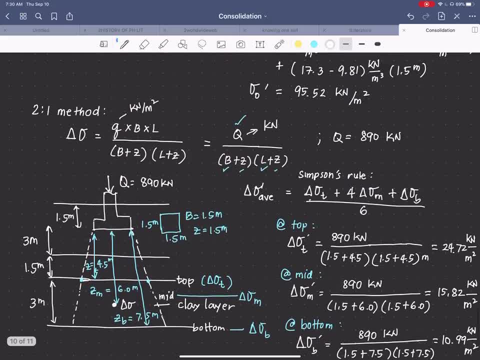 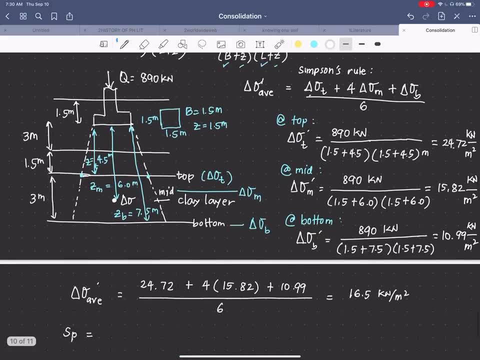 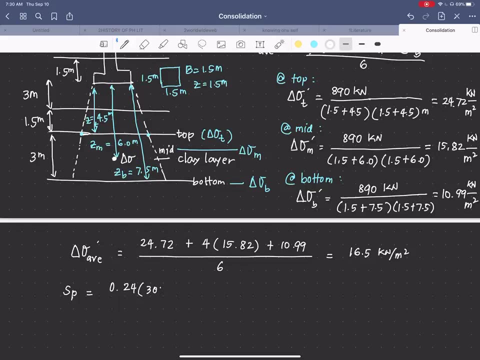 Primary consolidation settlement is equal to C sub C. Let's go back and look for our C sub C value, which is 0.27 here. So we have 0.27.. The thickness of the clay layer is 3,000 divided by 1 plus. 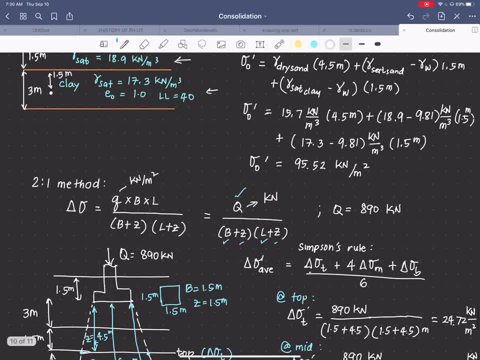 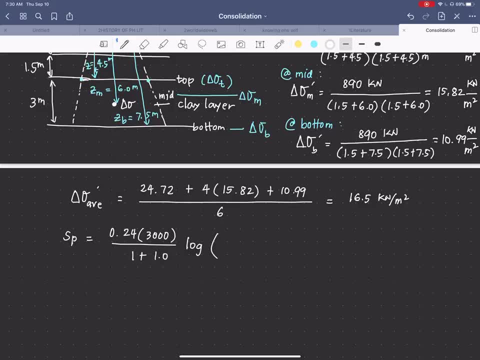 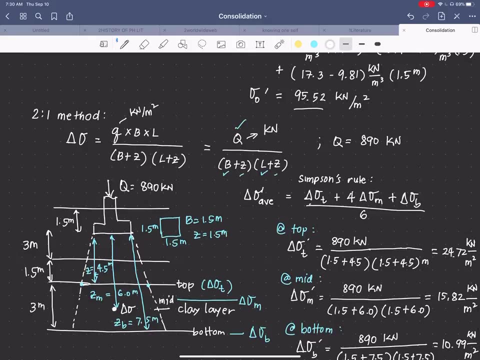 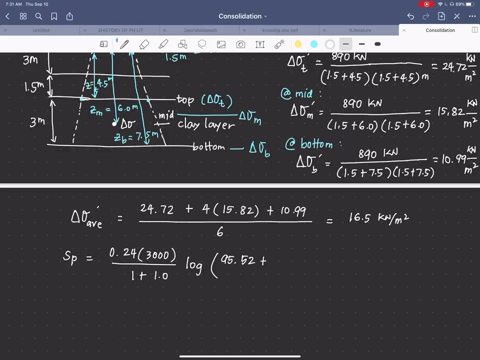 Our void ratio is 1 here, 1.. And then we have log of the effective stress- Let's go back again- which is 95.52.. 95.52 plus our surcharge of 16.5, all over 95 point. 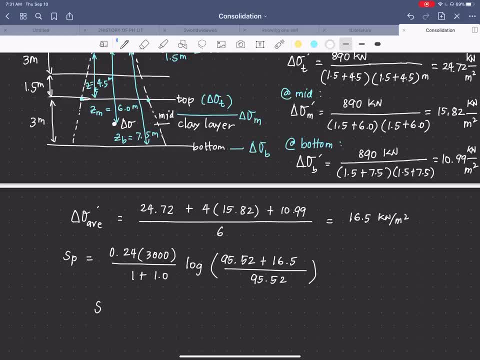 So from here, we can solve for our primary consolidation, which is equivalent to 28 millimeter. So that is our final answer. Thank you, Thank you. 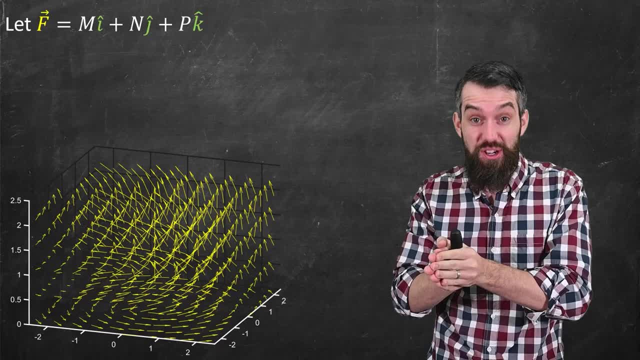 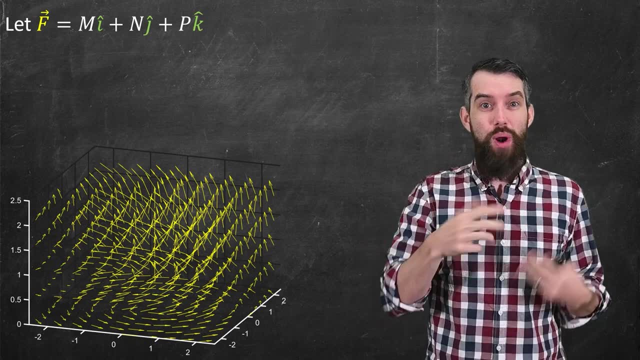 In this video we're going to talk about the curl of a vector field. This video is part of my full course in vector calculus and the playlist for that is down in the description. Now what I want to begin with is just some vector field in three dimensions, a vector field with three different. 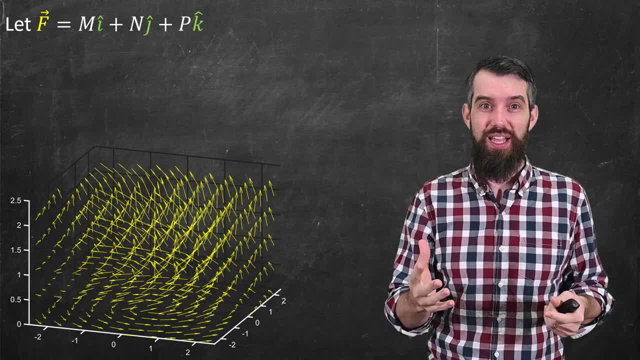 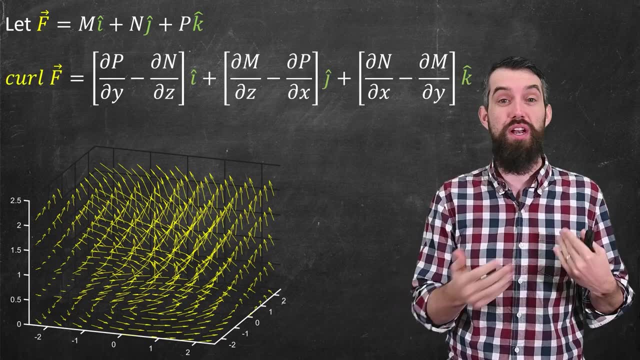 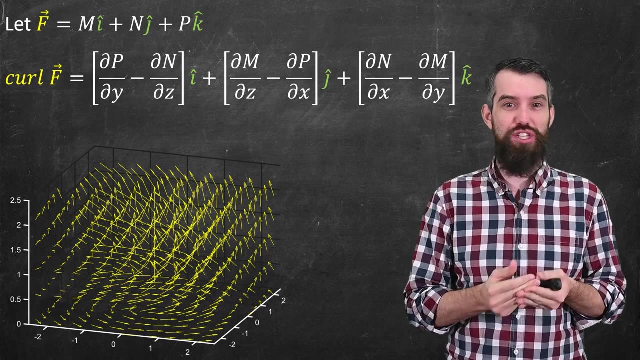 components and it looks like some sort of swirly mess. And then I'm going to define the following thing: This is called the curl of a vector field and it's written curl of just the vector field f. And well, it looks like a relatively messy algebraic expression and, don't worry, In a few 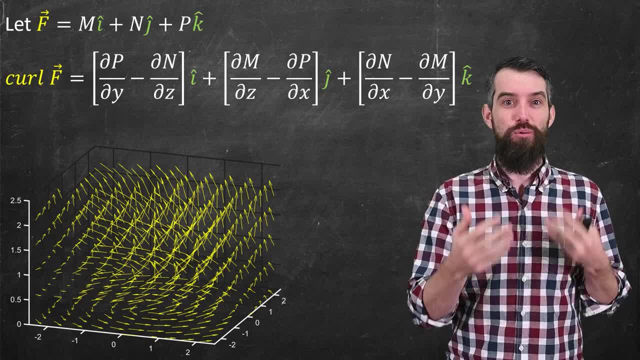 minutes. we're going to do something to clean it up and make this look a lot simpler, But right now, this is how it's defined. It's a vector. It's got an i-hat, a j-hat and a k-hat component. 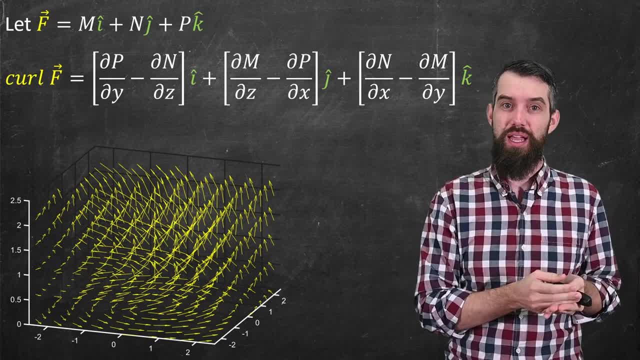 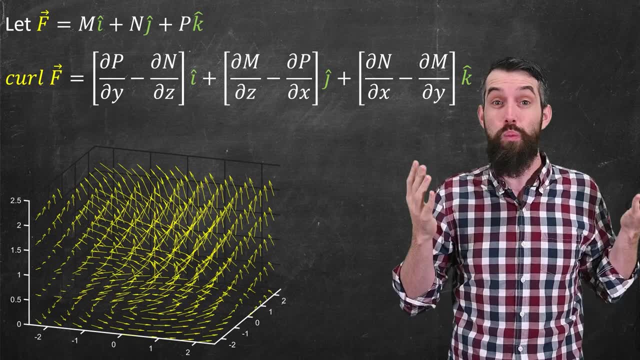 Each of those vectors is a difference of two different partial derivatives And basically, if you give me some vector field f, I can give you another vector field, the curl of f. But what does that mean? Now, when you look at this expression, there might be some part of it. 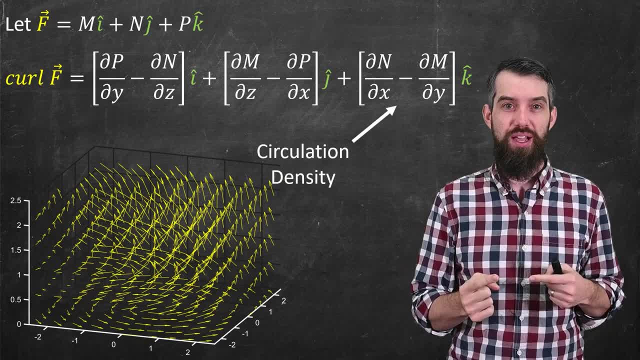 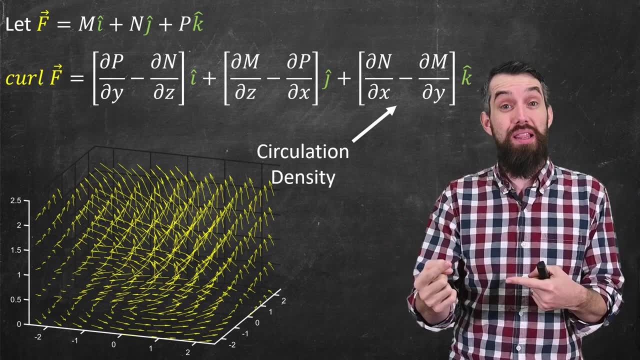 that you have seen before, in particular, the third component. We saw this back when we were talking about circulation, circulation density and the relationship between them that was expressed by Green's theorem. This was all something that we did in the two-dimensional